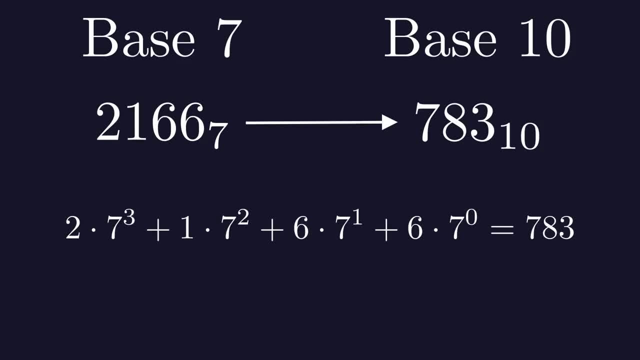 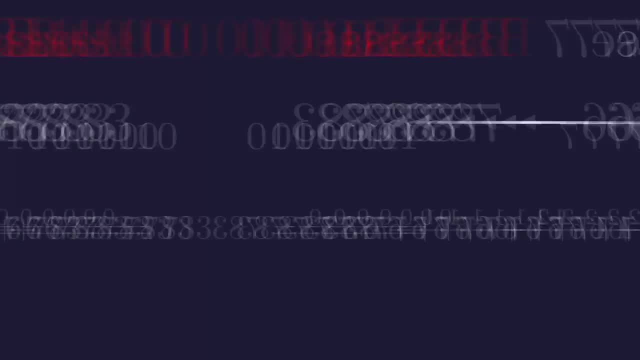 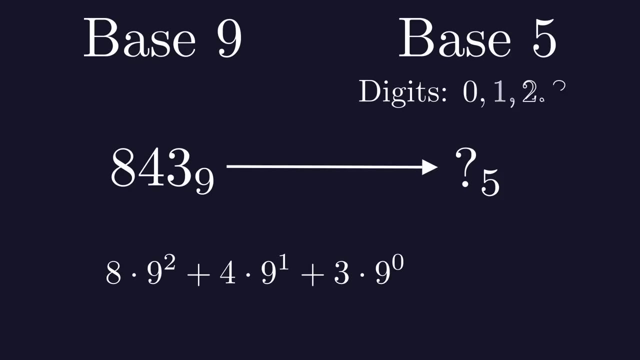 and add them all up. But there is one important thing we need to remember: When we want to convert a number to a base different than 10, we need to perform calculations in that base. In this example, we convert a number from base 9 to base 5.. In base 5 we can use digits from 0 to 4, so we have to write: 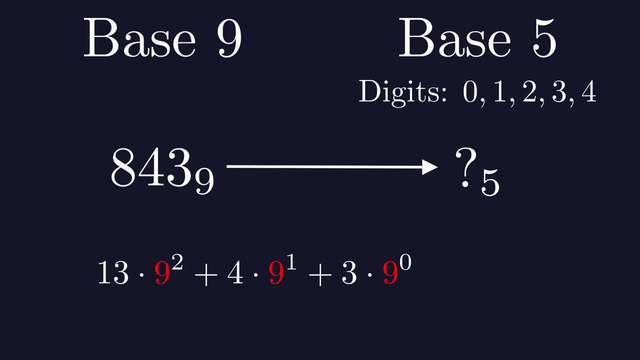 8 as 13 in base 5, and we also have to write 9s as 14.. Now we just multiply each digit by the corresponding power and add them up, But not forgetting that we make all calculations in base 5.. So 4 times 14 is equal to 1 to 1, and not 56 like in base 10.. One last thing before we talk. 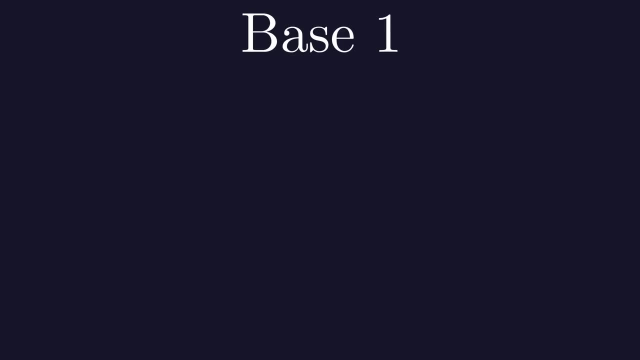 about negative number bases, The special case of base 1.. According to the rule that the other natural number bases obey, that in base b we use digits from 0 to b-1, in base 1 we would only be able to use digits 0, so we wouldn't be able to express. 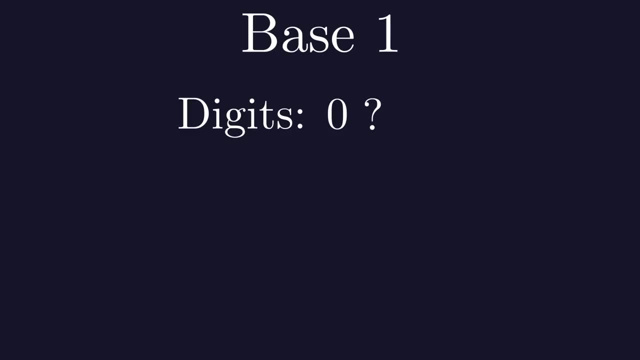 any value except 0. So to be able to express integers in this base, let's assume that we can use any sign as the only digit. This base isn't very efficient in expressing bigger values, because the value of a number is also equal to its length. When we talk about number bases, there's 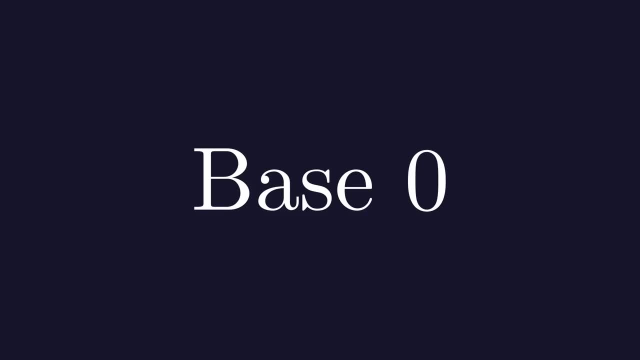 one that cannot be a number base and that is 0.. 0 raised to any integer is just equal to 0, and 0 raised to the power of 0 is undefined. So base 0 can't exist because it wouldn't be able to express. 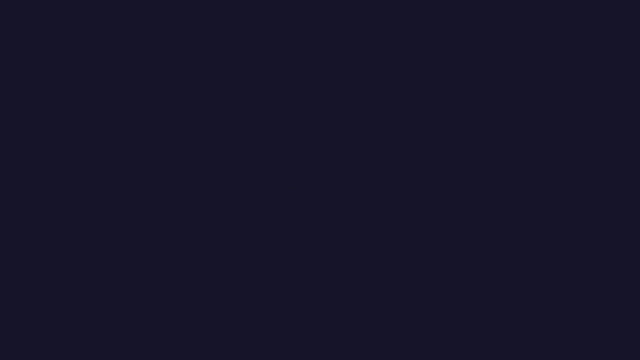 any value except 0.. Surprisingly, all other real numbers that you can think of can be a number base and all those bases can express integers. So let's start exploring those unique number bases from the negative numbers In base minus 10 digits represent different powers of minus 10.. 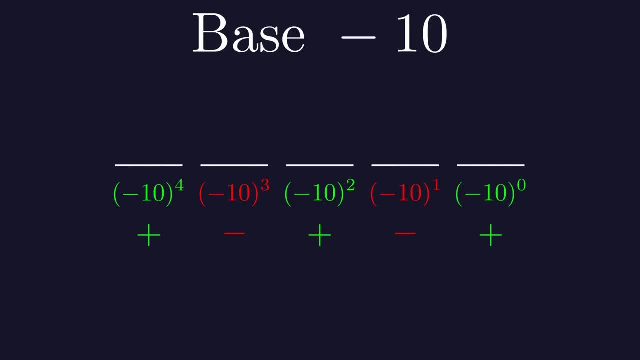 Odd powers are negative and the even powers are positive. But what digits should we use in this base? In positive number bases, we use digits from 0 to base minus 1.. To be able to express all integers in negative number bases, we will use digits from 0 to the absolute value of the base. 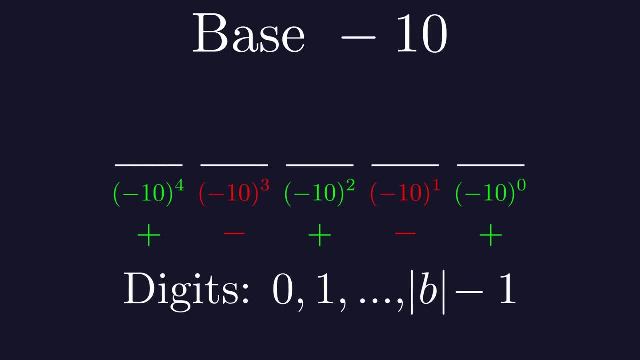 minus 1.. So in base minus 10 we will use the same digits as in base 10.. But the numbers written in base minus 10 don't look like those in base 10. Because the odd powers of minus 10 are negative. 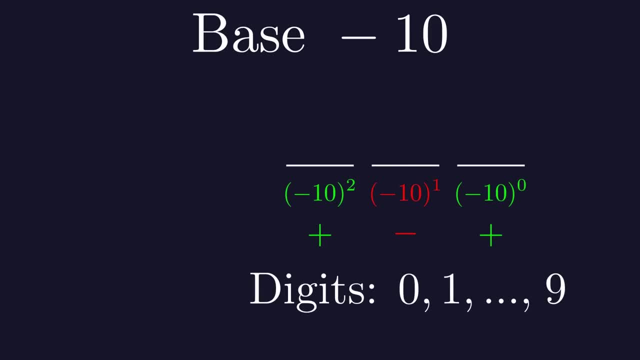 and this base are built differently. For example, to express 473 in base minus 10, we first have to take 5 hundreds, then add 3 minus 10s and add 3 units In base minus 10. we also can express negative values without using the minus sign. For example, this number is equal to minus 95.. All negative. 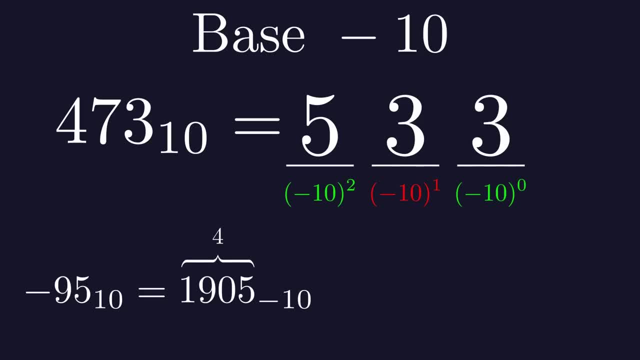 values have an even number of digits when they are written in negative base and all positive values have an even number of digits. Number bases of different negative integers behave like the base minus 10.. After integers we have rational numbers. Rational numbers are all fractions where the 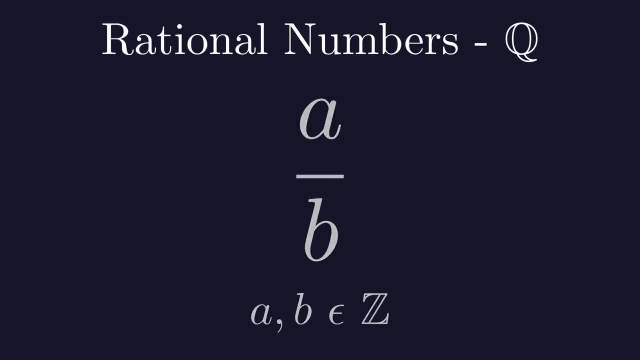 denominator and the denominator are integers. First let's look at bases of form 1 over some integer n, For example base 1- third. In this base digits represent different powers of 1- third, That is 1, 1 third, 1 ninth and so on. But if we write the decimal, 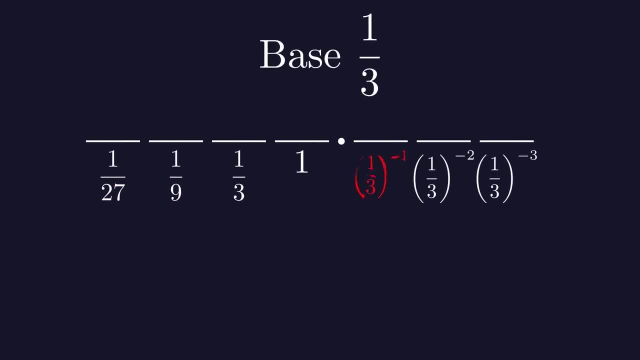 point. we get negative powers Which give us 3,, 9,, 27 and so on. All those values are just powers in base 3, but reversed, So to be able to express any number in base 1. third, we only need the same. 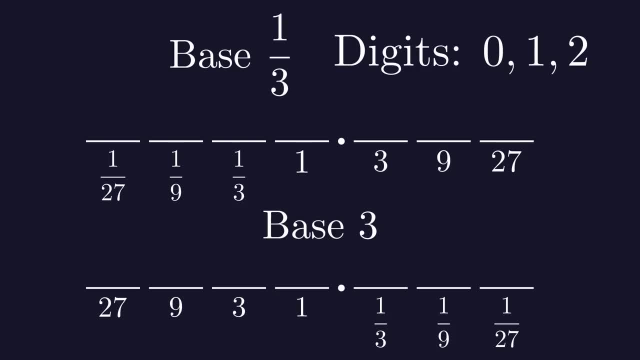 digits as in base 3.. So 0,, 1 and 2.. And also numbers written in base 1 third are just reversed numbers in base 3.. For example, 32 and 2 thirds in base 3 looks like this: So in base 1 third. 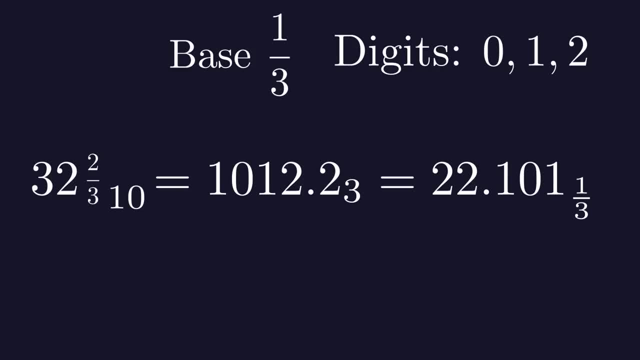 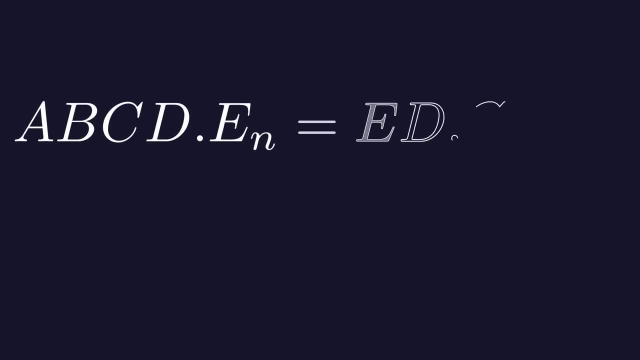 is written like that, And that is true because after multiplying the digits by the corresponding power of 1 third, we get 32 and 2 thirds. That is true for any base that is of form 1 over some integer n. Another fact is that in all bases of form 1 over some integer n, we use digits from 0. 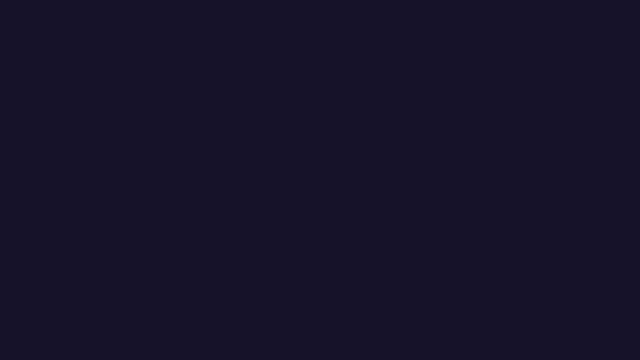 to the absolute value of n minus 1.. Now let's look at the fractions of form a over b, where a and b are not equal to 1.. First let's see the example where a is bigger than b, For instance base 7 thirds. In this base, as in all other bases, digits represent different. 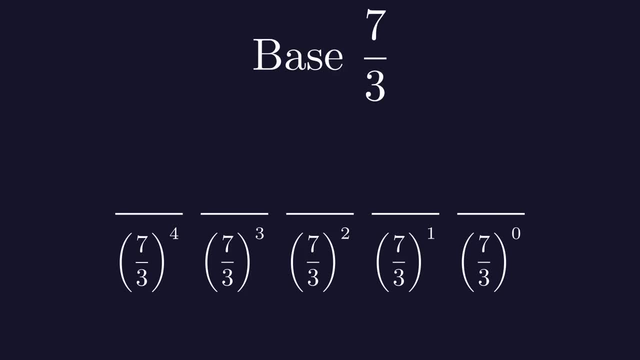 powers of 7 thirds. But what digits should we use? Because we have 7 in denominator. let's first take a closer look at base 7.. To convert numbers to base 7, we can just multiply each digit by the corresponding power and add them all up, Not forgetting that we have to perform all calculations. 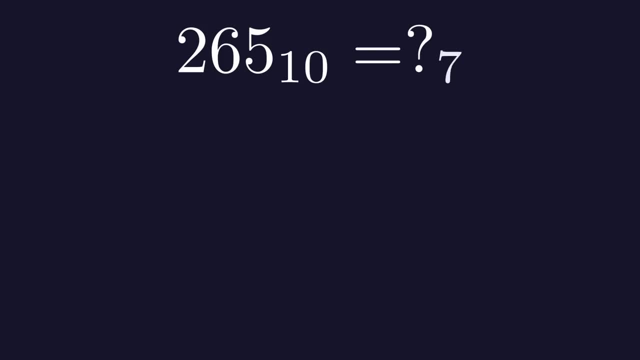 in base 7.. But there is a faster way that allows us to convert numbers between bases. Let's say that we want to convert 265 to base 7.. First we divide 265 by 7. We get 37 and a reminder. 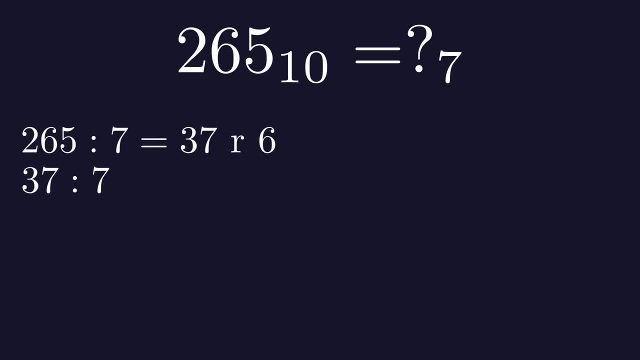 of 6.. Then we divide 37 by 7. We get 5 and a reminder of 2.. Now we divide 5 by 7. We get 0 and a remainder of 5.. It means that 265 in base 7 is written as 5 to 6.. Why does this method work? 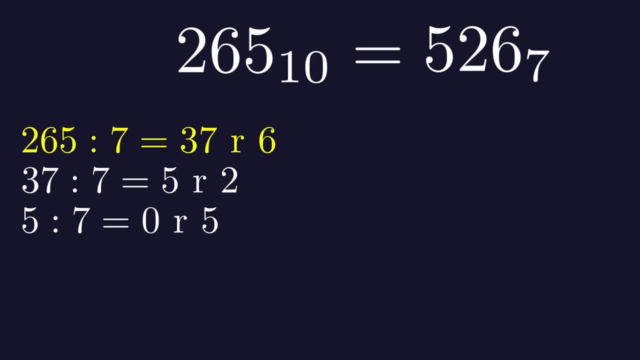 And we get 37 with a reminder of 6.. That means we can write 265 as 37 times 7 plus 6.. Next we divide 37 by 7. So 37 can be written as 5 times 7 plus 2, Entering a limit of 37 plus 2 after solving the previous case. 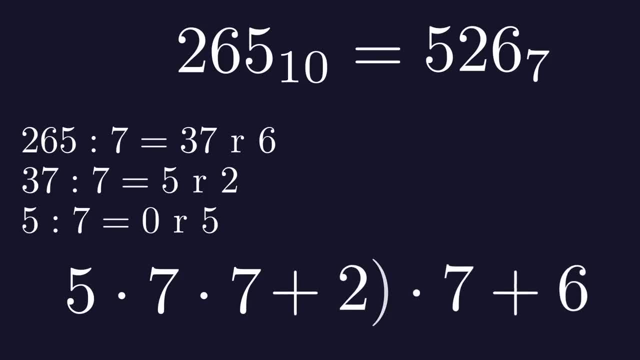 After multiplying everything out, we get that this is equal to 5 x 7 x 7,, which is equal to 7 to the power of 2, plus 2 times 7 to the power of 1, and plus 6 times 1,, so 7 to the power of 0. We quite simply took four times 2 x 7.. Now let's see how would this work in base 7.. In base 7, it has a r sl Hawaiianран box. I will just write the 0 product and give 0 to the number of numbers. but i'm making for something different. 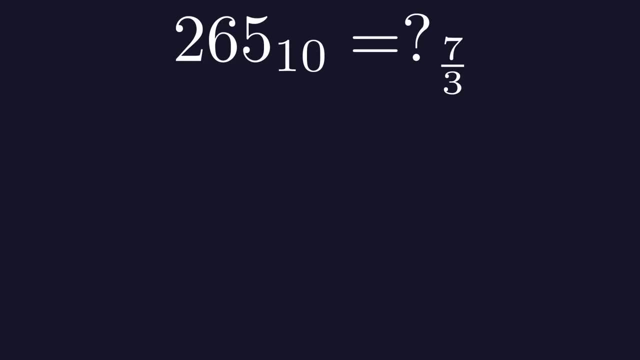 Let's first look at this example with thisink value in base 7.. Let's say, compared to 1 and b, how would this work in base 7? thirds? We start the same. We divide 265 by 7.. Now we do something. 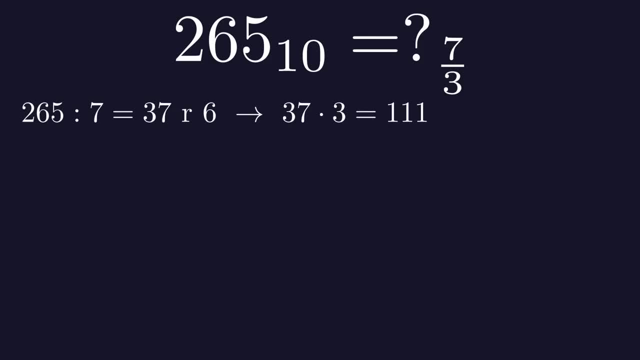 different. We multiply 37 by 3.. Then we divide 111 by 7. We get 15 and a remainder of 6. So we multiply 15 by 3 and divide by 7. We do it until we get 0. It means that 265 in base 7 thirds looks. 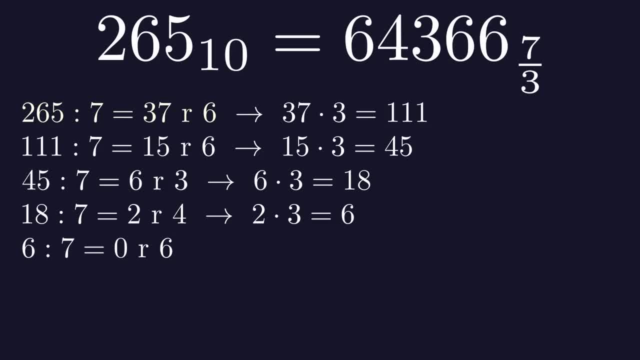 like this. And again, why does it work? We divided 265 by 7, so we can write it as 37 times 7 plus 6.. Then we multiply 37 by 3. It means that we can write 37 as 111 divided by 3.. We can write it: 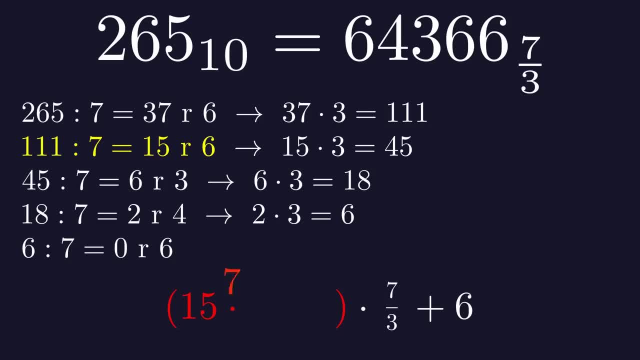 like this: Then we can write 111 as 15 times 7 plus 6.. Then we can write 15 as 45 divided by 3.. And so on. After multiplying everything out, we get this. So we know that this is a representation of 265. 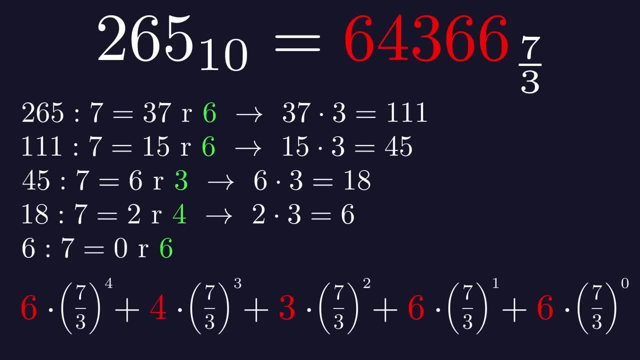 in base 7 thirds, Because the digits are the remainders. when we divide by 7, we know that in base 7 thirds we can use digits from 0 to 6.. This trick is really useful when we want to convert numbers to fractional bases, But it only works if the denominator is bigger than the denominator. 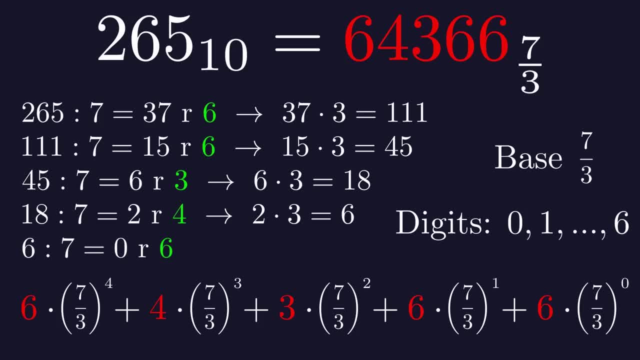 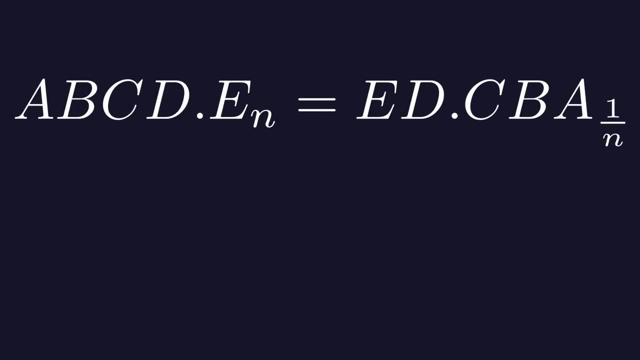 But now let's look at number bases where the denominator is bigger. We have already seen that numbers written in base 1 over n are just reversed numbers written in base n. It also means that numbers written in base a over b are reversed numbers written in base. 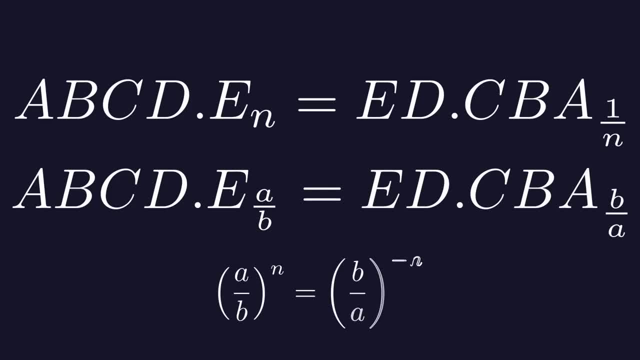 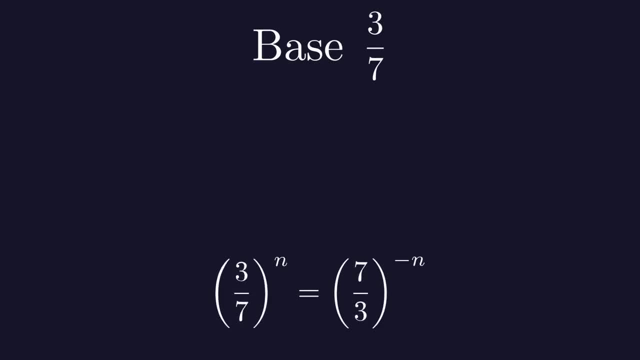 b over a, because a over b to the power of n is equal to b over a to the power of minus n. Let's look at base 3 sevenths. the reverse of 7 thirds. 265 was written as 64366 in base 7 thirds. 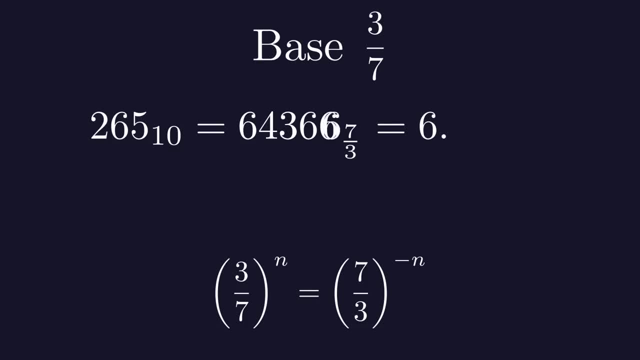 So in base 3, sevenths, it will be written as 6.6346.. And we can see that this is true because after multiplying the digits by the corresponding powers and adding them up, we get 265.. So in this base we will also use digits from 0 to 6.. 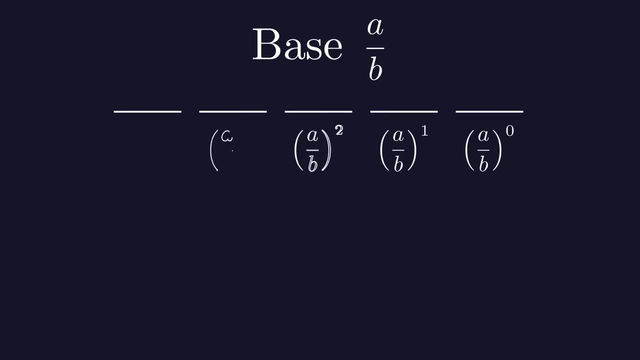 To sum up: in base a over b digits represent different powers of a divided by b. If a is bigger than b, we use digits from 0 to a-1,, but if b is bigger than a, we use digits from 0 to b-1.. 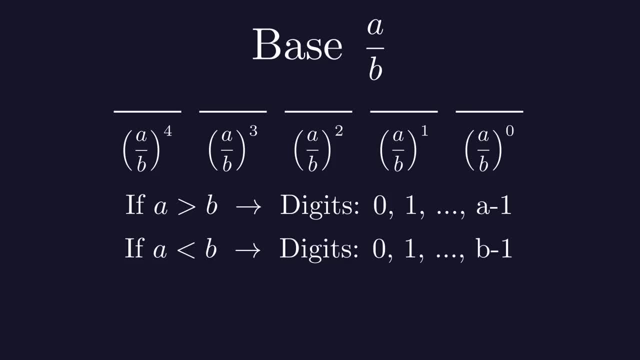 And if we want to convert the number to base where b is bigger than a, we first convert this number to base b over a and reverse it. The real numbers, apart from containing rational numbers, also contain irrational numbers. Those are numbers that can't be expressed as a ratio of two integers. 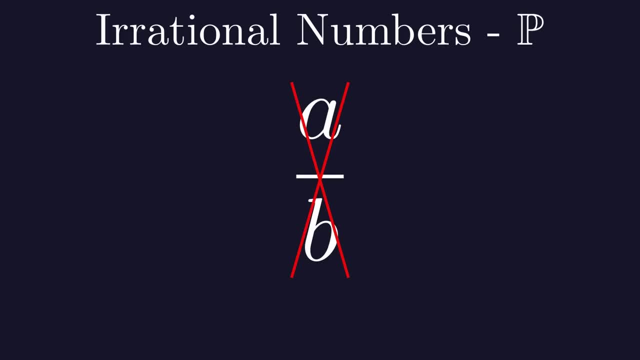 So in this case the real numbers are numbers that can't be expressed as a ratio of two integers And, written in base 10, have an infinite decimal representation, For example the square root of 2, the cube root of 5, or pi. 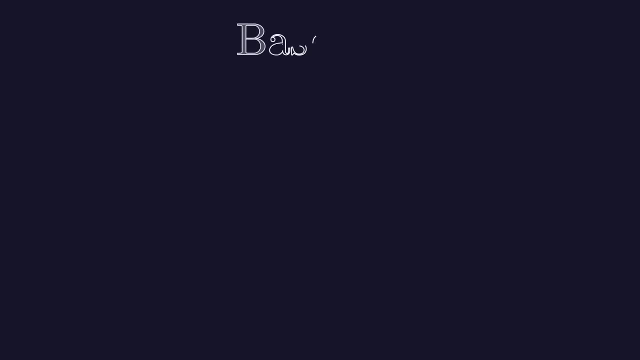 First let's look at number bases of square roots. For example, base square root of 5.. In this base, digits represent powers of the square root of 5.. This base has a lot in common with base 5, because the square root of 5, raised to the 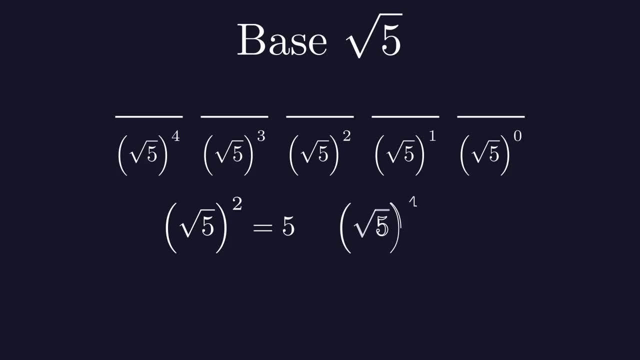 power of 2 is equal to 5.. The square root of 5 raised to the power of 4 is equal to 5 to the power of 2.. In general, the square root of 5 raised to the power of 2n is equal to 5 raised to the. 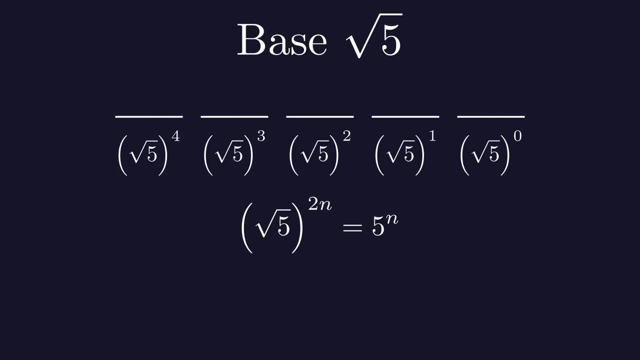 power of n. So to express any number in base square root of 5, we only need to use the same digits as in base 5, that is, from 0 to 4.. For example, 97 in base square root of 5 is written as 30402.. 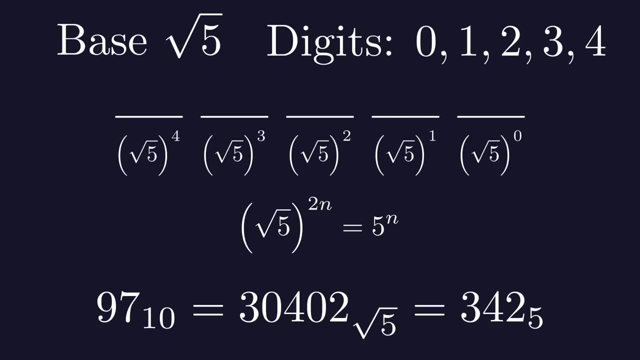 This number, represented in base 5, is just 342.. The digits that represent odd powers of the square root of 5 are all equal to 0. This will be true for any rational value, But in this base we can also easily express irrational values that are multiples of square. 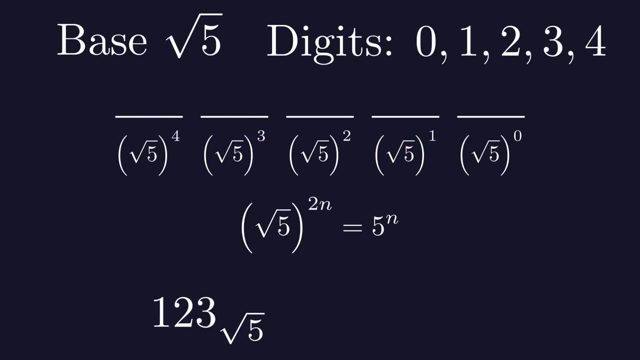 root of 5.. For example, 1 to 3 in this base is equal to 8 plus 2 times square root of 5.. Here the digits representing the odd powers are not equal to 0. With the same logic we can create number bases of higher roots. 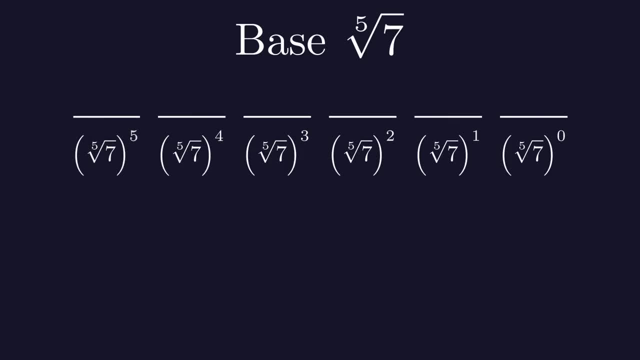 For example, the fifth root of 7.. Fifth root of 7 to the power of 5 is equal to 7.. And generally, The fifth root of 7 to the power of 5n is equal to 7 to the power of n. 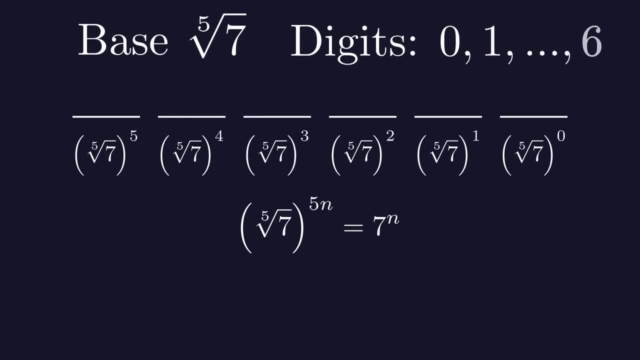 So with this base we can use the same digits as in base 7.. 36 in base 7 is represented as 5: 1. To express this value in base fifth root of 7, we just have to write zeros where the powers of the fifth root of 7 are irrational. 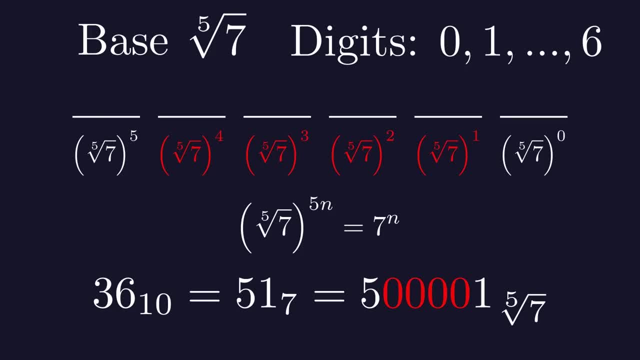 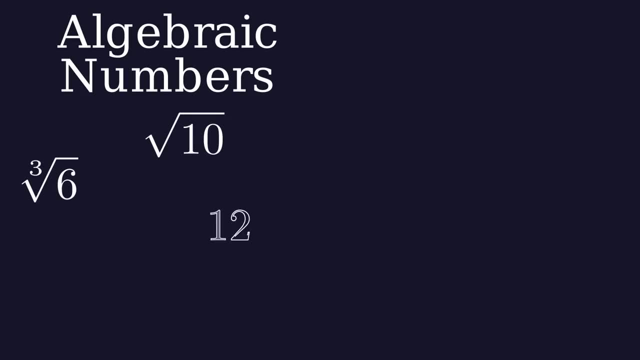 Like this we can create a number base from any root of any number. All roots are algebraic numbers, Which means that they can be a solution to a polynomial With rational coefficients. But irrational numbers also include transcendental numbers Like pi or e. 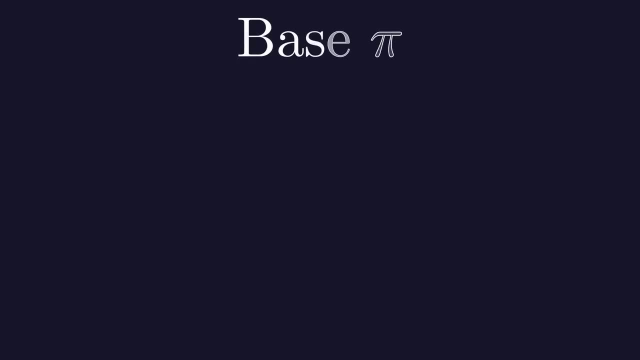 Let's see how base pi works. In base pi, digits represent different powers of pi, But it isn't clear what digits should we use. Maybe the same digits as in base 3. Because it is the closest integer to pi. But then the only integers we would be able to express in this base would be 0,, 1 and. 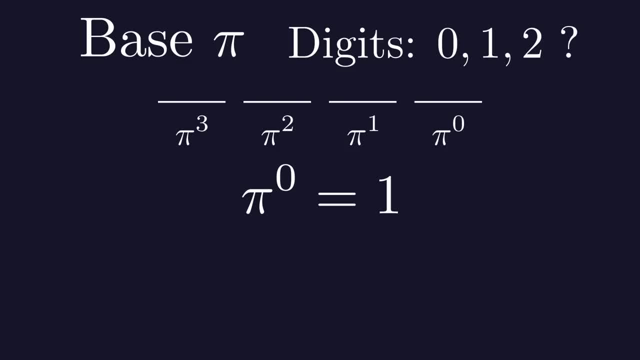 2. Because only pi to the power of 0 gives us an integer, And that's it. Just as pi in base 10 has an infinite decimal representation, 10 in base pi would also be infinite, As would all other integers. 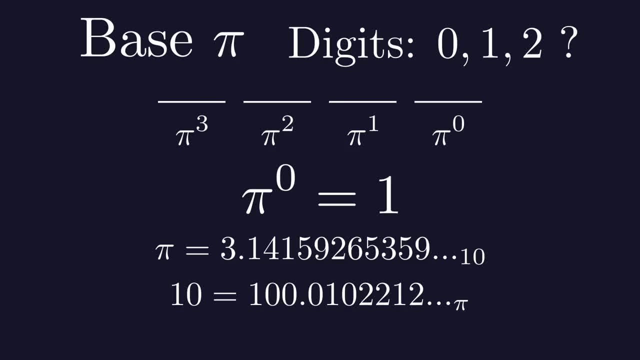 So theoretically it is possible to create base pi, but it doesn't work as good as algebraic number bases. The same is true for the number e, Which is also transcendental, But surprisingly base e is special in a way To explain why we first need to talk about radix economy. 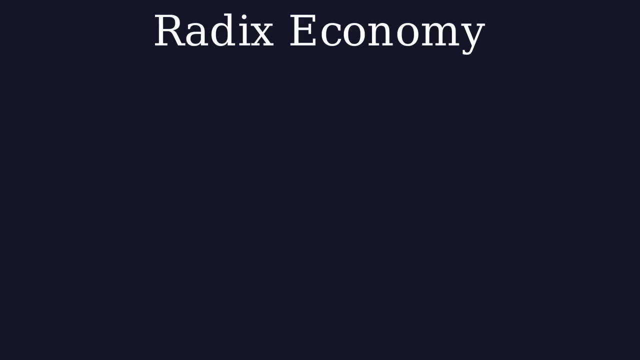 Radix economy is a way to measure efficiency. Radix economy is a way to measure efficiency. Radix economy is a way to measure efficiency of a number base. For example, in base 16, we can write all values between 0 and 255 using only 2 digits. 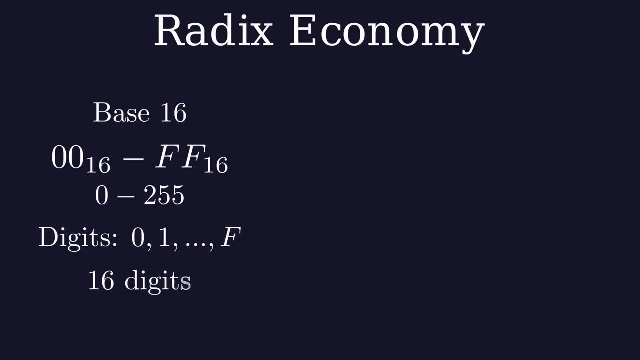 But in base 16 there are 16 possible symbols each digit could have. On the other hand, in base 2 we have only 2 possible symbols each digit could have. But to express all values from 0 to 255 we would need 8 digits. 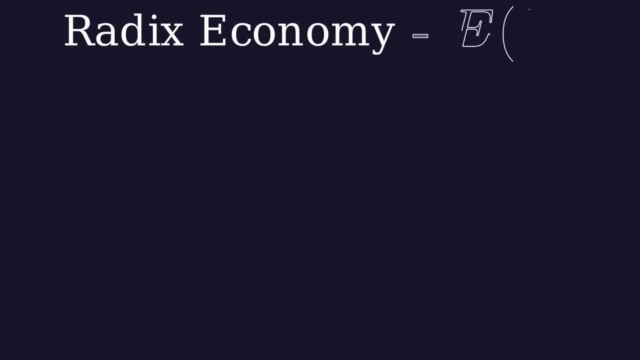 The radix economy is calculated for a number written in some base. For example, To calculate the radix economy for a number- 231- written in base 10, we take the number of digits used to write that number. In this case it is 3.. 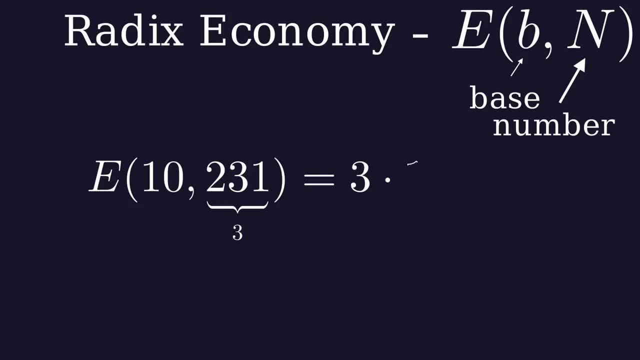 And multiply it by the total number of symbols in that base, In this case 10.. So the radix economy of the number 231 written in base 10 is equal to 30.. Radix economy for a number n written in base b can be generalized by this formula: 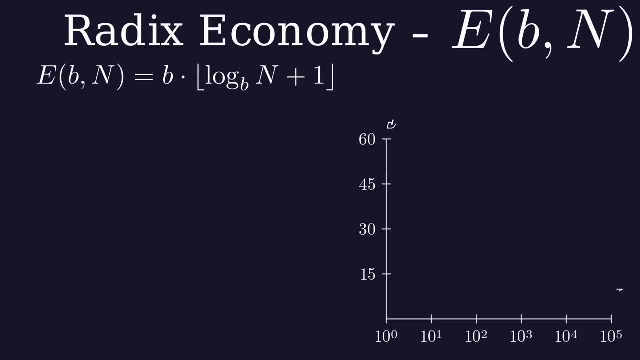 We can graph this formula for b equal to 10.. And the horizontal axis is in the logarithmic scale. We can see that the function jumps when we add a new digit, But when n gets very large the jumps become less and less significant. 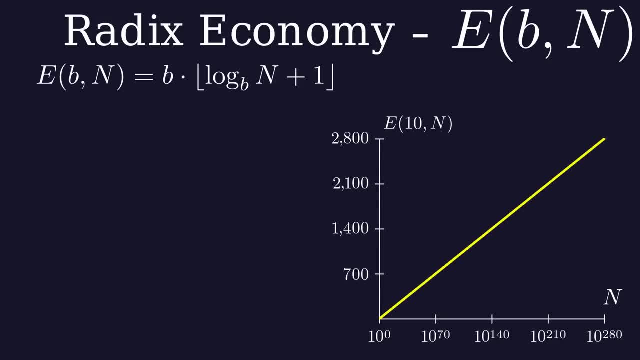 Which means that for large values of n, this formula can be approximated by b times log of b of n, And that is equal to b times ln of n divided by ln of b. So if we want to know which number base has the smallest radix economy, we just need to. 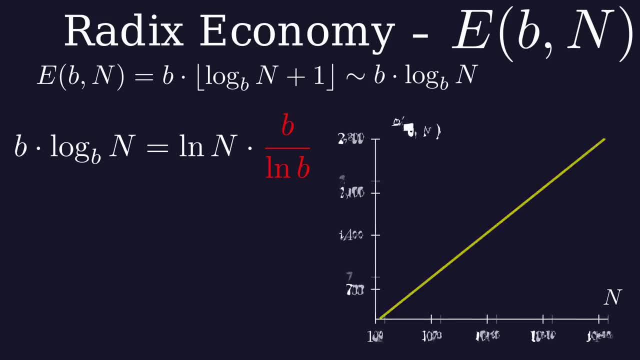 know for what b this part is the smallest. We can graph this function and we can see that it has a minimum at the number e. So it means that base e is the most efficient number base. But, as we have seen with base pi, transcendental numbers don't work so well as bases. 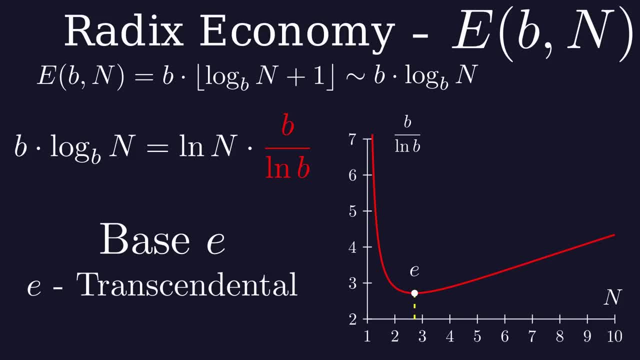 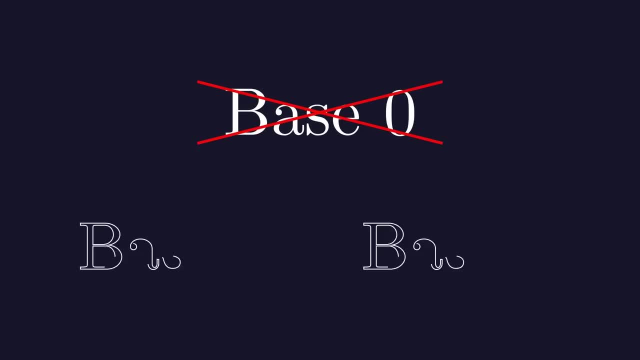 So this information isn't very useful, and it's here just as a fun fact. So we now know that all real numbers except 0 can be a number base, Although some of them do not work as good as others. Outside the real numbers, 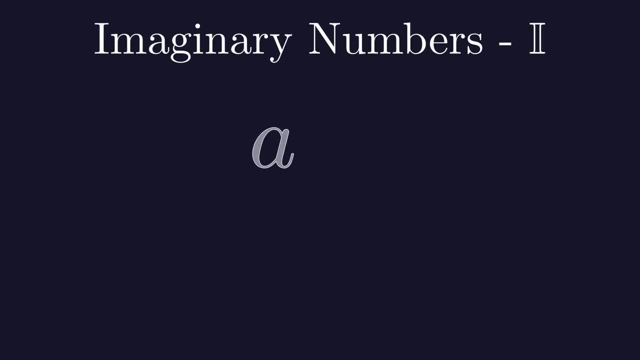 We have imaginary numbers. Imaginary numbers are real numbers multiplied by the imaginary unit i, Which is equal to the square root of minus 1.. We can create number bases using imaginary numbers, and they can even express both real and imaginary numbers. For example, base 3i. 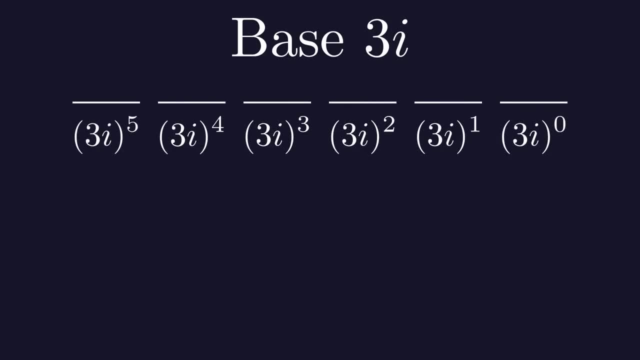 In this base digits represent different powers of 3i. 3i to the power of 0 is equal to 1.. 3i to the power of 1 is equal to 3i. 3i to the power of 2 is equal to minus 9.. 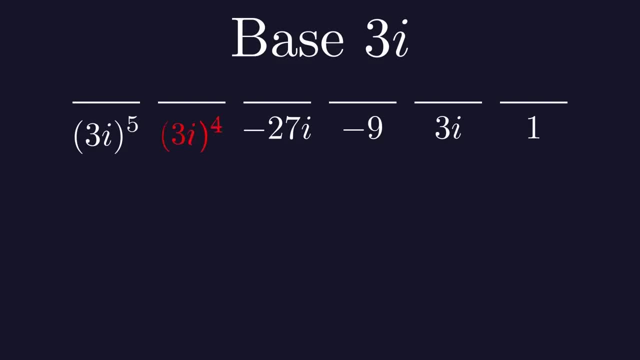 3i to the power of 3 is equal to minus 27i, And so on. This creates a pattern where you have a positive real number, then positive imaginary number, then negative real number, then negative imaginary number and then again positive real number. 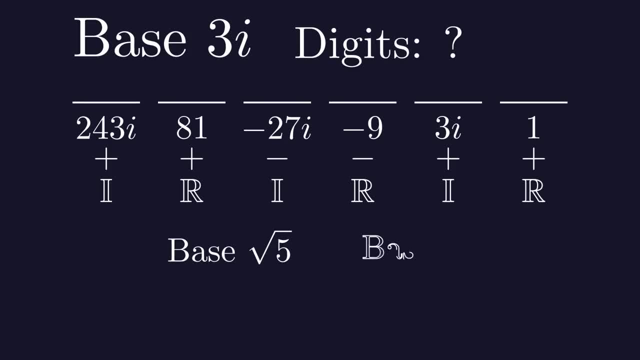 But what digits should we use in this base? In base square root of 5, we use the same digits as in base 5.. 3i is equal to the square root of minus 9.. So in this base we will use the same digits as in base minus 9.. 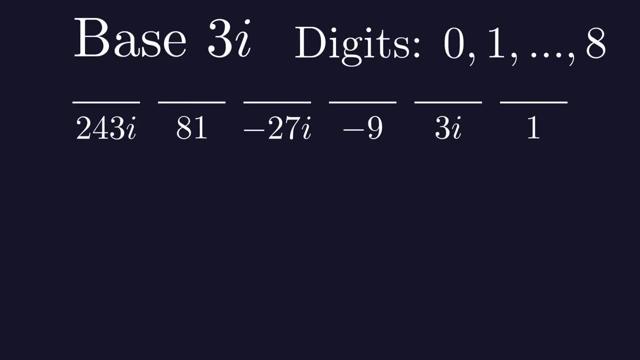 That is 0 to 8.. This allows us to express any real and any imaginary number, But this base also allows us to represent numbers that have both the real and the imaginary part. For example, 72 in this base is equal to 21 plus 2i. 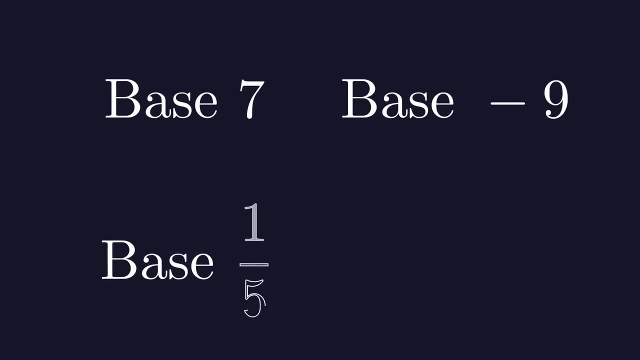 As we have seen, we can create number bases from almost all real numbers and pure imaginary numbers, But unfortunately we can't create number bases from all complex numbers. For example, let's look at base 2 plus 2i. In this base, the digits represent different powers of 2 plus 2i. 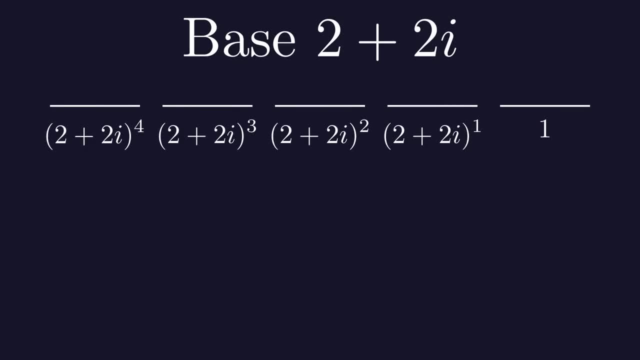 2 plus 2i to the power of 0 is equal to 1.. Then we have just 2 plus 2i, then 8i, and so on. Any number to the power of 0 is equal to 1.. 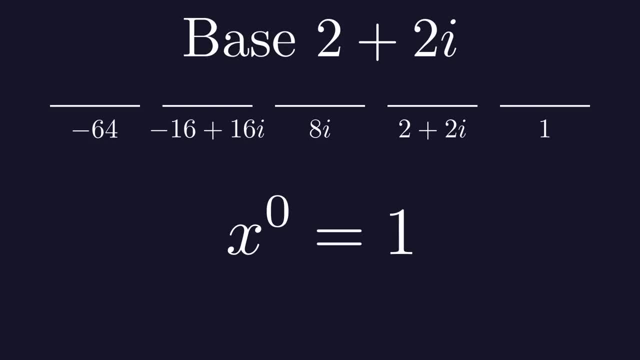 That allows us to express all integers in any base if we use the right digits. But in complex number bases we also want to express all complex numbers. Here the smallest multiple of i is 2.. So we are only able to express multiples of 2i. 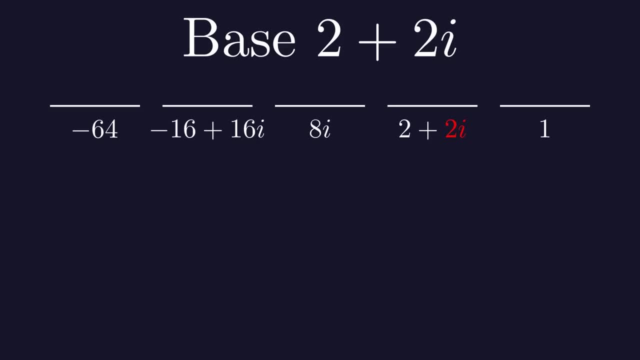 We can't express any odd multiple of i in this base. When we wanted to express any multiple of i in a pure imaginary number base, we could just use negative powers. For example, in base 3i we had powers 1, 3i minus 9, and so on. 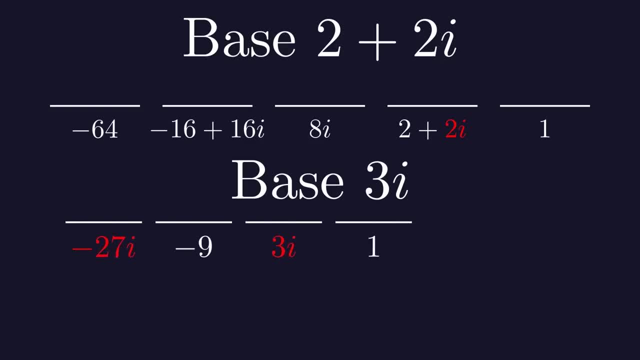 And all other powers were a multiple of 3i. But 3i to the power of minus 1 is equal to 1 over 3i And when we multiply denominator and the denominator by 3i we get that this is equal to minus i. 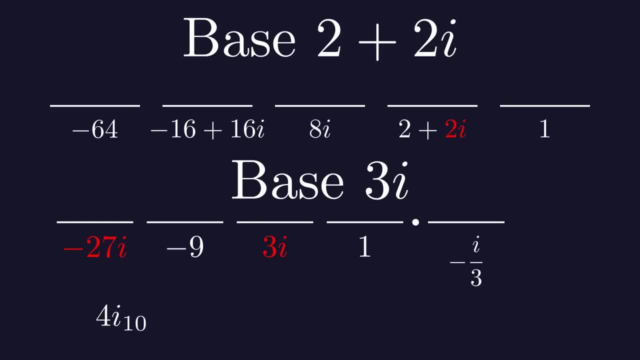 over 3.. So if we wanted to write 4i in this base, which is not a multiple of 3i, we could just take 2 times 3i and 6 times minus i over 3.. So 4i expressed in base 3i would be 20.6.. 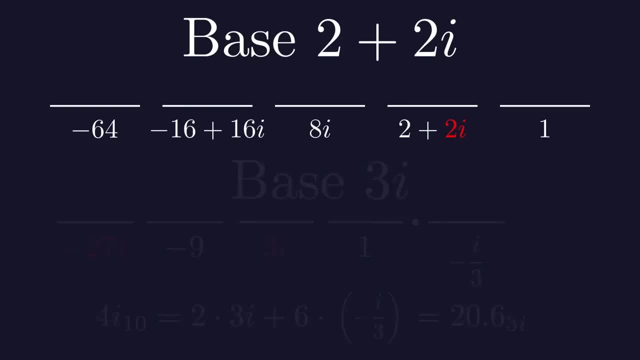 So to be able to express all imaginary numbers in complex bases, they need to be of form n plus or minus i. But that is not the only problem. Let's look at base 1 plus i. In this base we can express odd multiples of i. 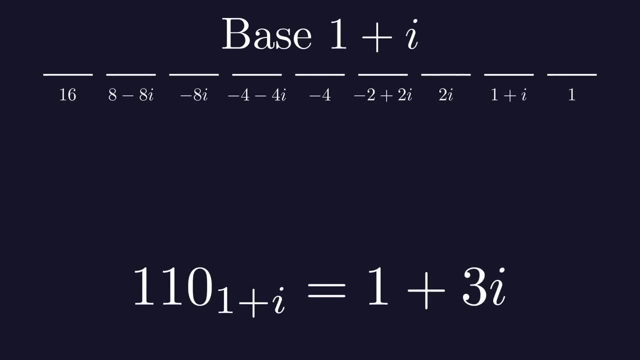 For example, 110 would be equal to 0. And n would be equal to 1 plus 3i. But let's look closer at the powers we can use. First we have a positive real number, Then positive real and positive imaginary. 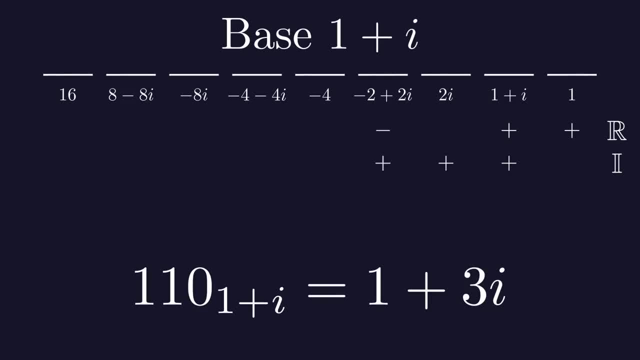 Then positive imaginary, Then negative real and positive imaginary, Then negative real, Then negative real and negative imaginary, Then negative real, Then positive real and negative imaginary. Then we again have a positive real and the cycle repeats. We can see a pattern here. 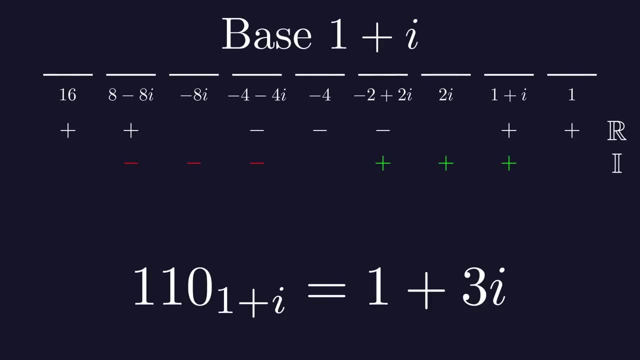 We have 3 positive imaginary values, three negative imaginary values. Then we would again have three positive imaginary values. Real values create the same pattern. To express all values in this number base we would need too many digits because we have so many positive values next to each other and so many negative. 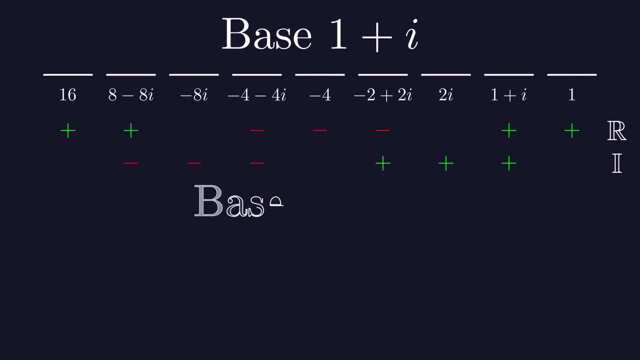 values next to each other. But now let's look at base. In this base, the pattern in powers is very different. Real and imaginary values alternate between positive and negative. This allows us to express any number using only digits 0 and 1.. But we only 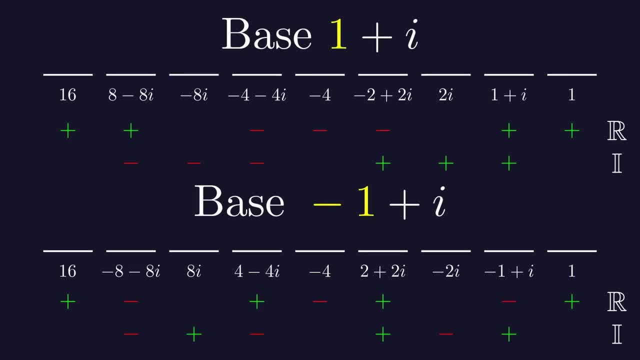 changed the positive one to negative one in the base. Let's see what happens when we change the i to negative. We can see that in base we still have a pattern where the positive and negative values are in groups of three, But in the second base we have a pattern where the positive and negative values alternate. 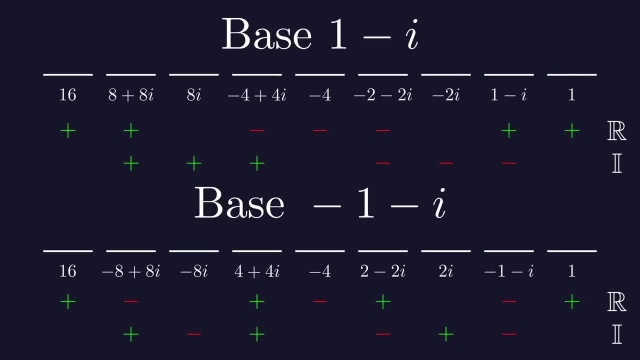 So the pattern doesn't depend on the sign of i, but it depends on the sign of real number. We can change one to any other natural number, For example base, and In the first base the positive and negative values are again next to each other In the 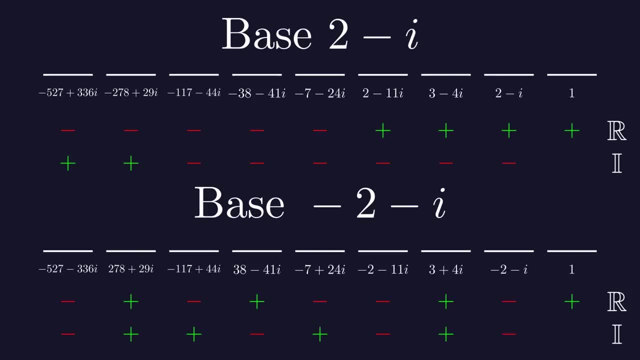 second base, positive and negative values are not exactly alternating, but they are not in big groups, and that will still allow us to express any number. So now we know that the complex number bases have to be of form plus or minus i, And to express any complex value in those bases we only need to use digits. 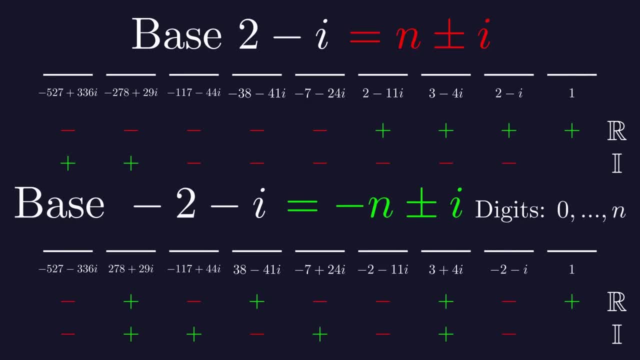 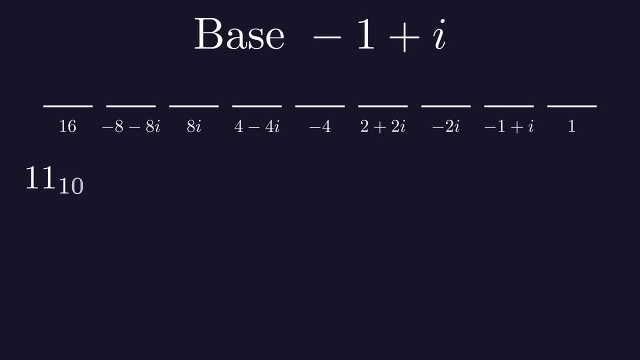 To see how this works, let's go back to base. In this base we can express any number with digits 0 and 1.. For example, to express 11,, we start with 16,. subtract 8 and 8i, add 8i. add 2 and 2i. subtract 2i and add 1.. 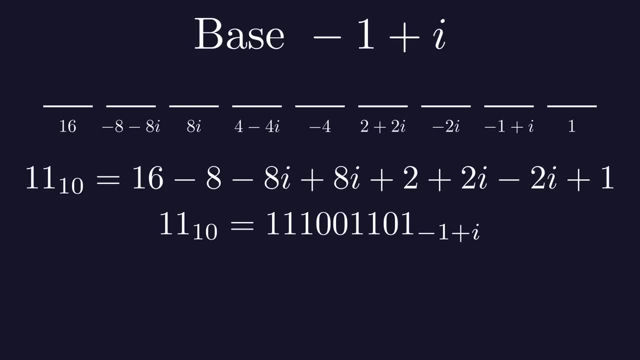 That's a complicated way to express 11.. But one thing the complex bases are good at is expressing imaginary and complex numbers with numbers Without the use of the letter i. For example, 7i expressed in this base would look like this: 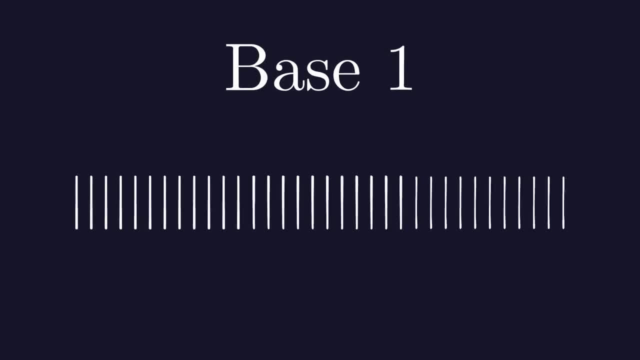 All those unusual number bases are interesting to explore. Some of them have advantages and some of them are just useless. So maybe to not overcomplicate things, we should stick to base 10 for now.